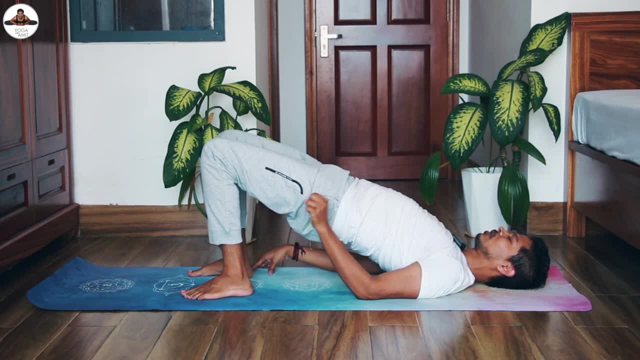 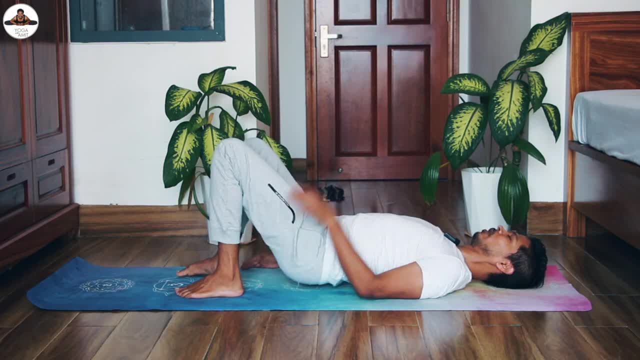 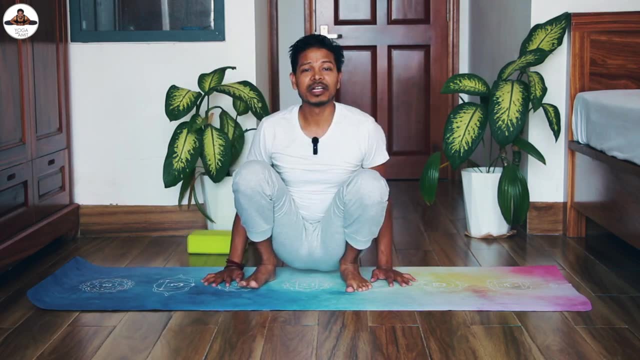 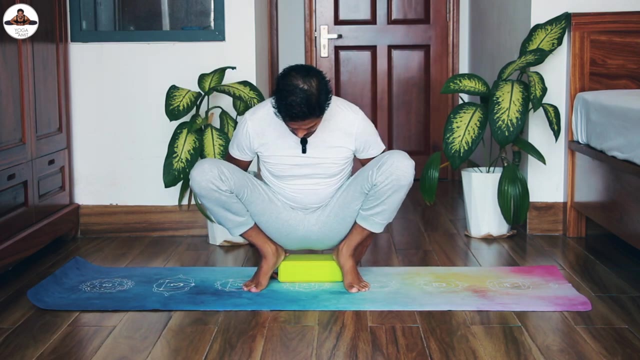 And then push with your hands. Sit up, Bring your feet flat on the ground. If you have difficulty sitting in a squatting position, take a block and place it under your knees, So you can put either under your knees like this. Let me show you from the side. 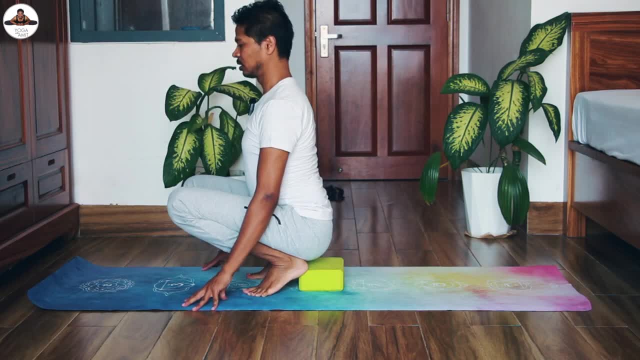 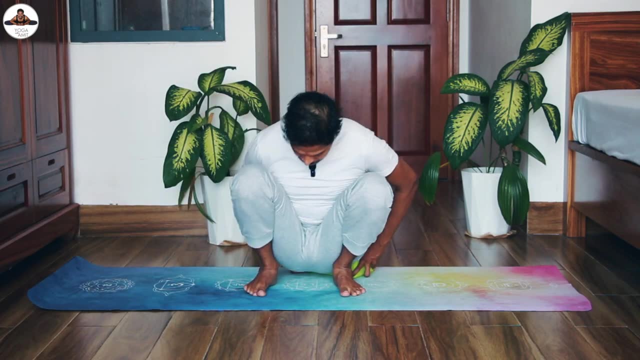 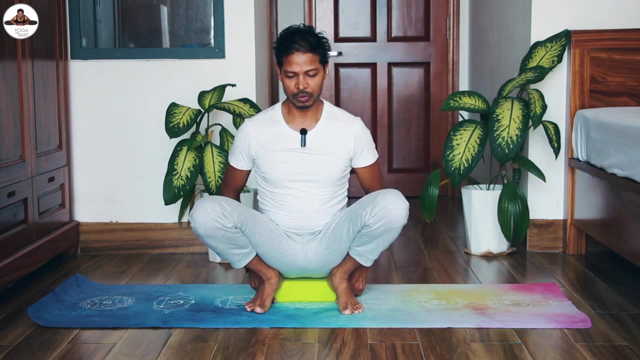 You take the block, place it under your heels. That will be easier and helpful for doing this asana. So let's place the block under block, or folded blanket under your heel, Or you can place your sitting bones onto the block, whichever feels the most convenient. 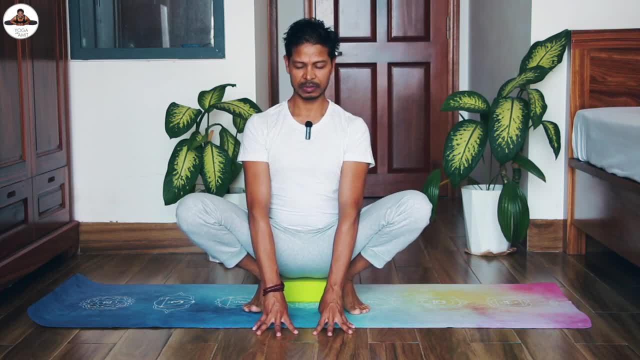 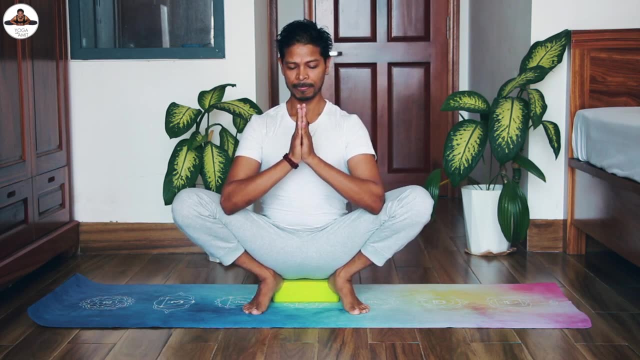 Lift your chest up using your hands and palm together, And you are opening the knees a little bit wider more. And then you're going to do the same. You are going to apply the Aswani Mudra, So you're going to squeeze the anus and release. 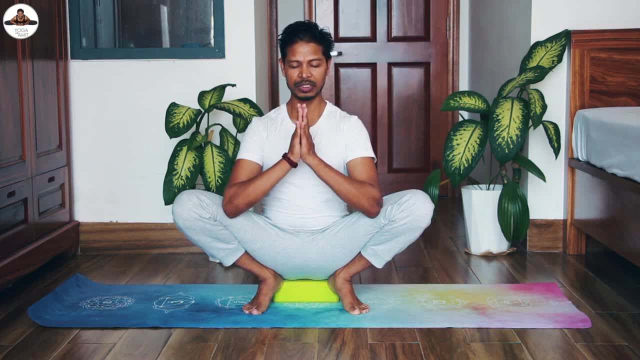 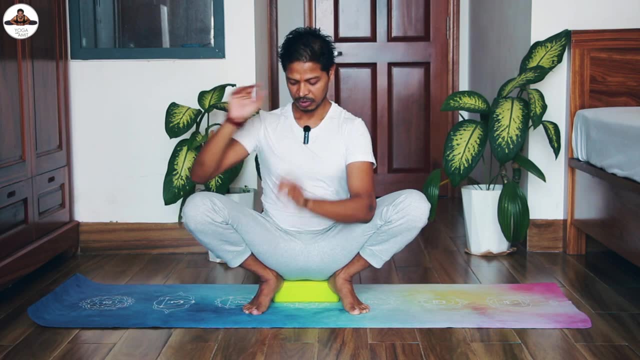 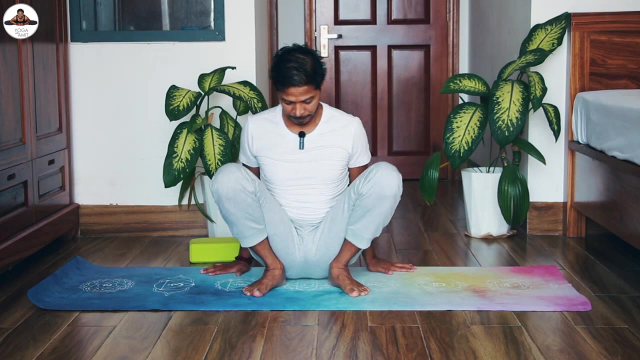 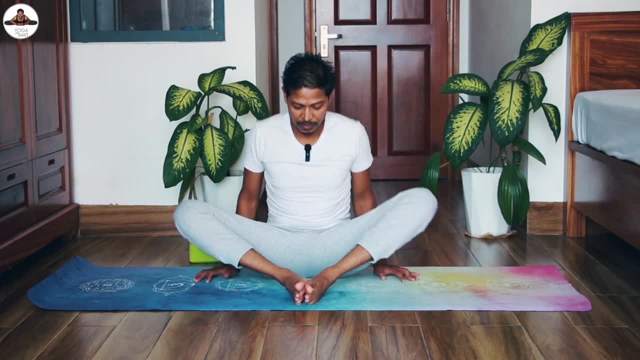 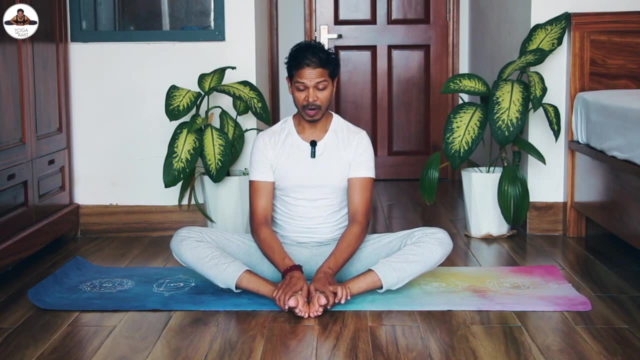 Then join the sole of the feet together and bring your feet wherever it feels most convenient. So check, do you need to have them far to be able to keep your back straight? Or when you bring the feet near, is it still your back straight? 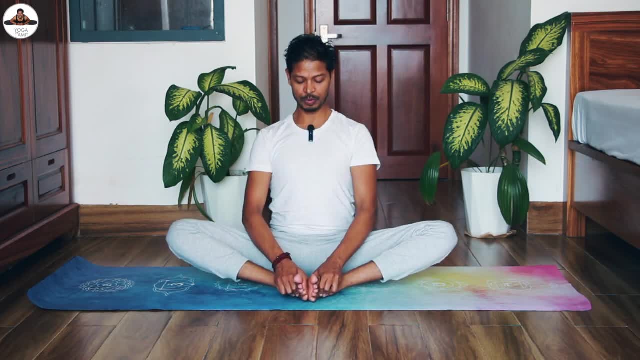 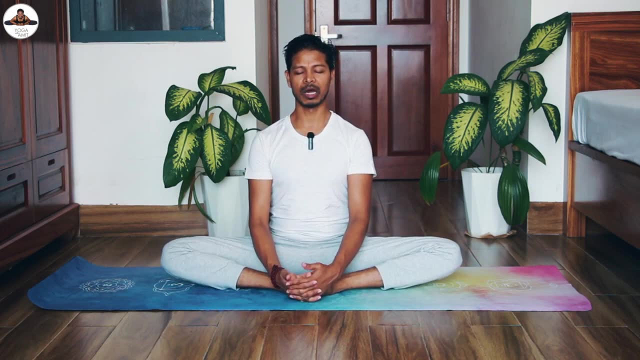 Because you don't want to bring the feet near and you're hunching. You want to keep your back straight. Then you try to press your knees down, as down as possible without any discomfort, And then, once again, we are going to apply the Aswani Mudra.